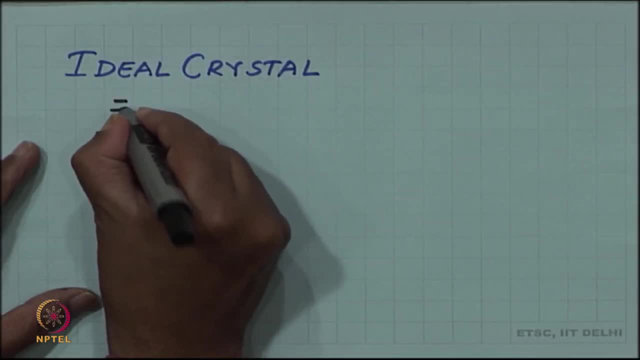 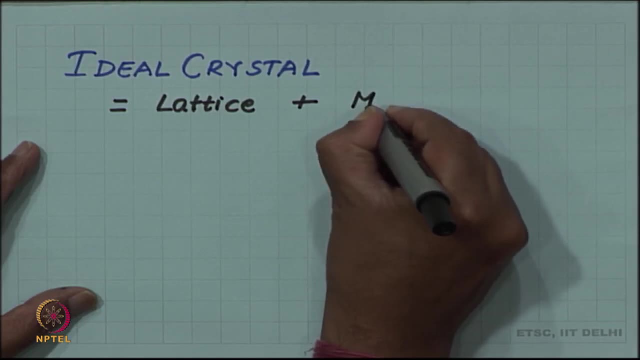 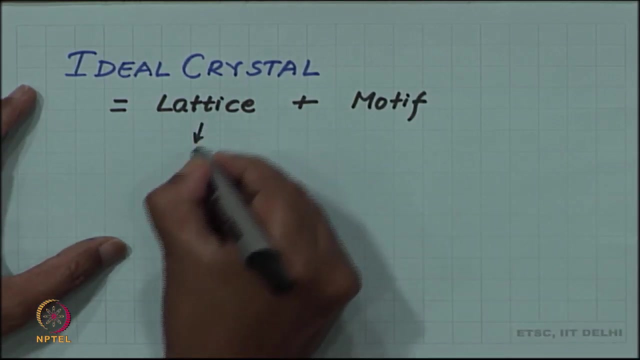 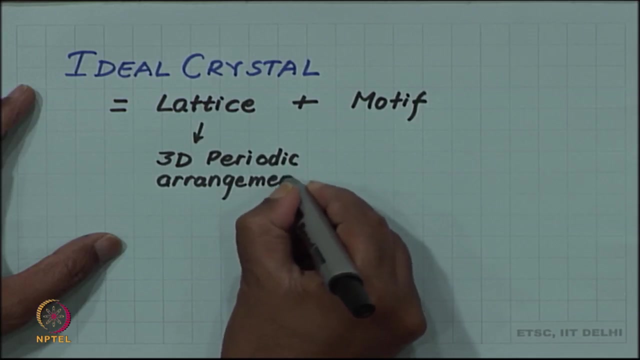 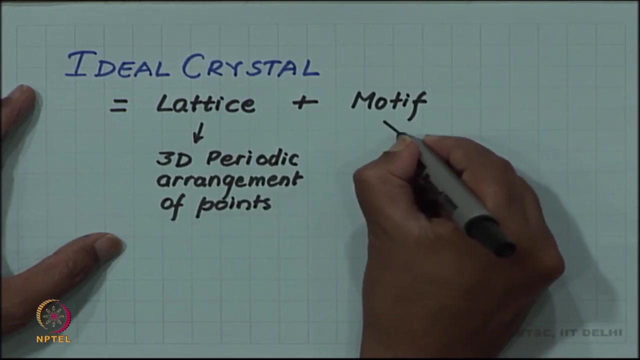 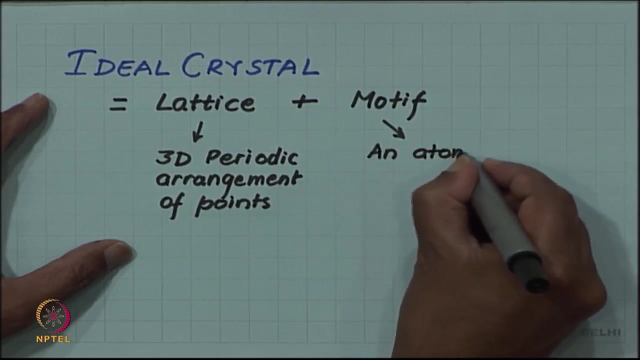 till now is the ideal crystal which we discussed in terms of lattice and a motif, And we said that the lattice was a 3D periodic arrangement of points, three dimensional periodic arrangement of points And motif. then on each of these points we put an atom or a group of atom associated. 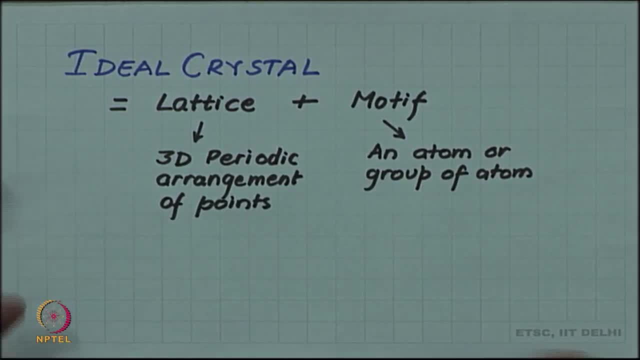 with each lattice point. So this was the theme And we develop this theme in great detail with the several examples we have seen. All those examples till now was of ideal crystal. These crystals were not supposed to have any defects. but then real crystals will show deviations from ideality. real crystals will 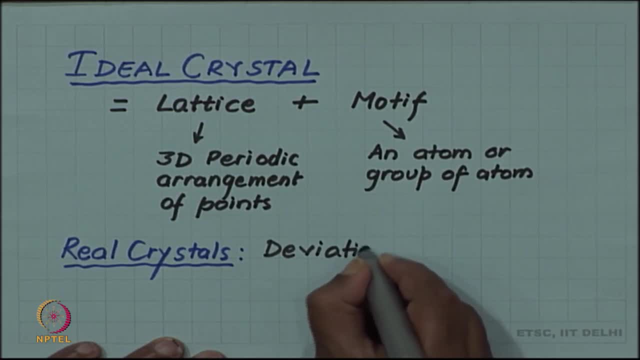 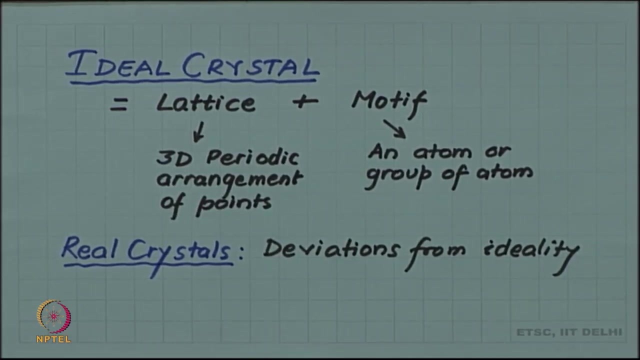 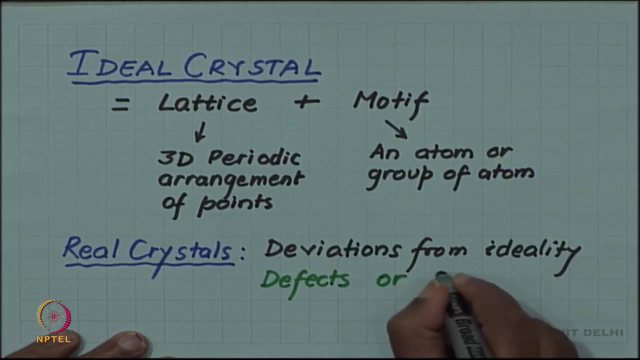 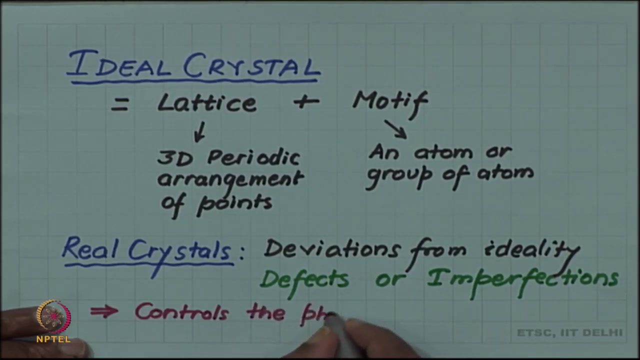 deviations from ideality. These deviations are what are termed as defects or imperfections, and they are very important topic in material science because these defects or imperfections control the properties of material, So they are very important in controlling both physical and mechanical properties. 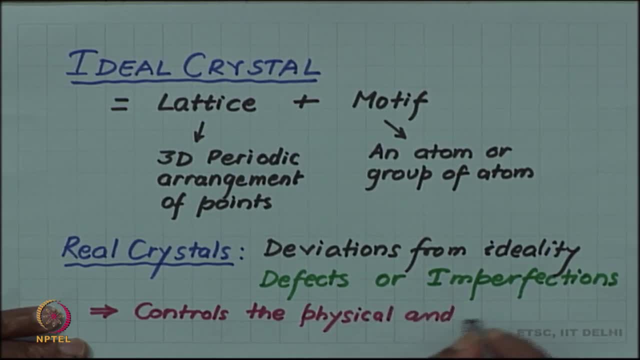 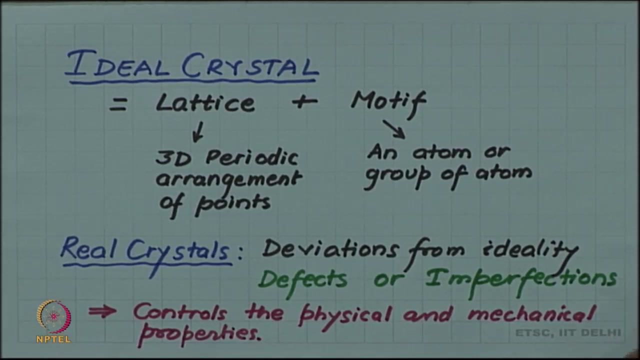 So it is important to have a serious study of defects in crystal, Of course, to study the defect. why we spent considerable amount of time in ideal crystal, It is that defect can always be with respect to deviation from ideality. So we have to. 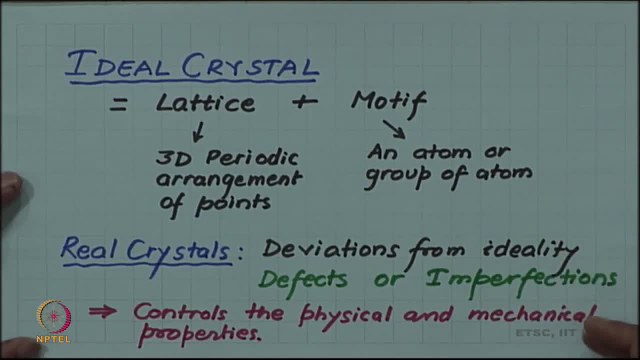 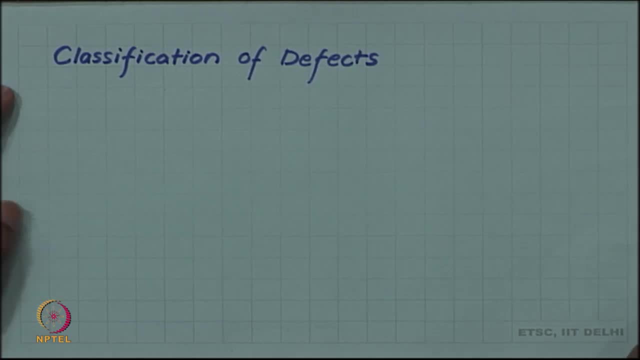 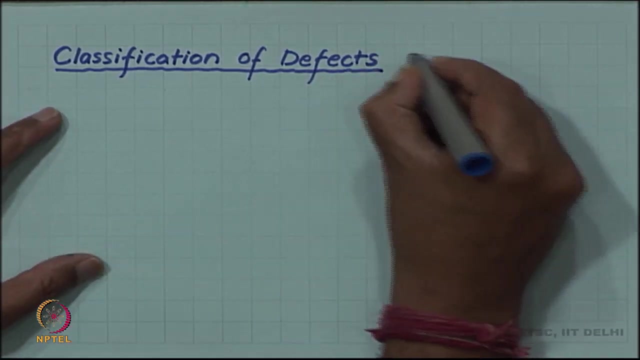 know what ideal structure we are talking about, then only we can talk about the defect or structure defect in the structure. Defects can be classified in one way of classification: is based on the dimensionality. So this classification which we are going to give you is based on. 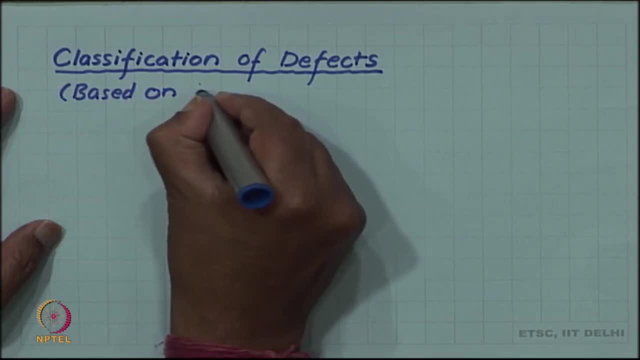 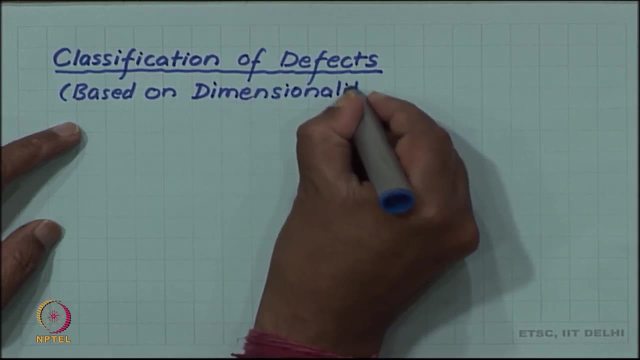 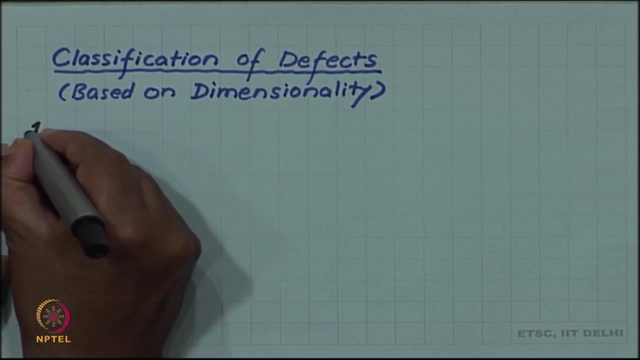 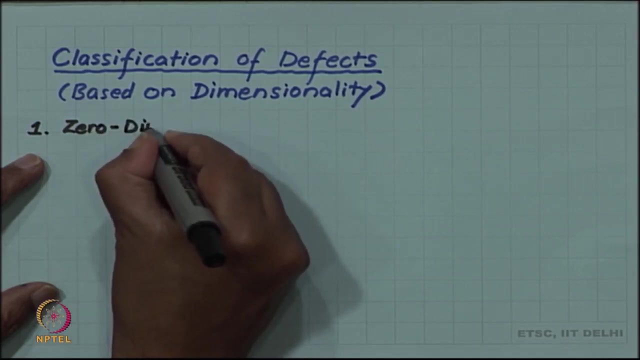 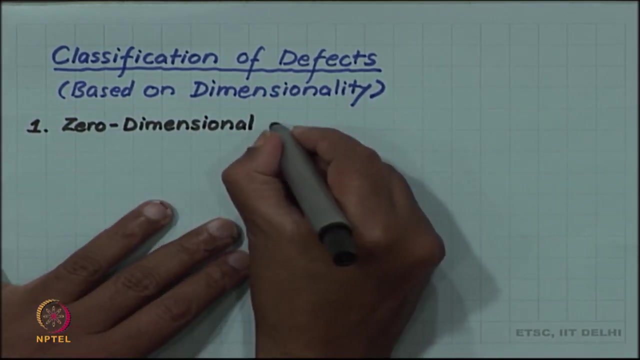 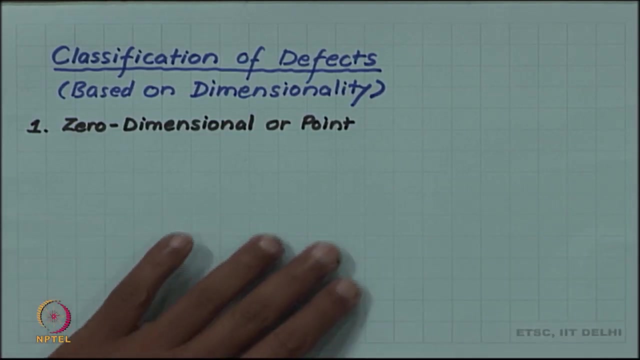 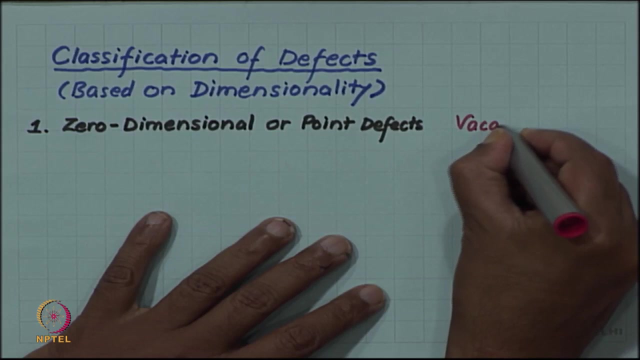 the dimensionality, So we can have zero dimensional. So this classification can be classified in one way, or can also be called point zero, dimensional or point defects. An example of such defects will be vacancy. Another example can be interstitial. 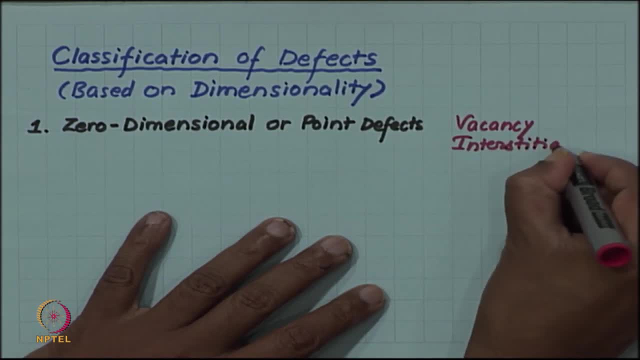 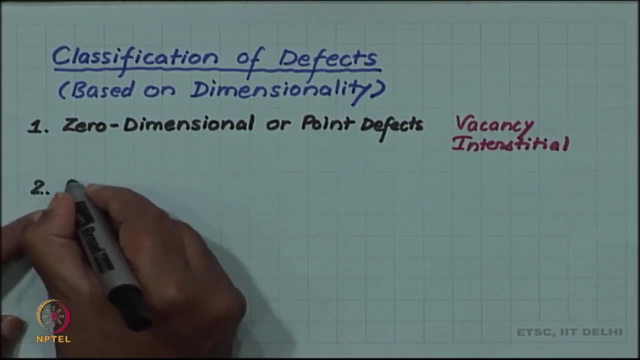 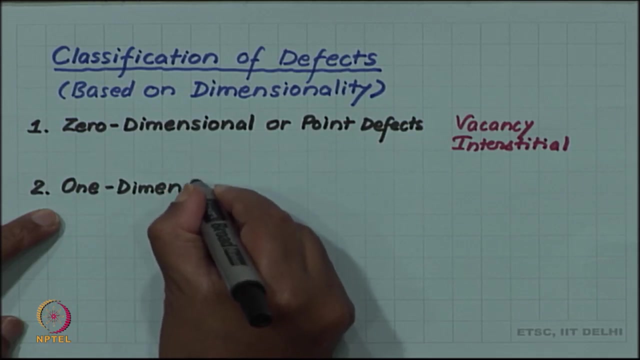 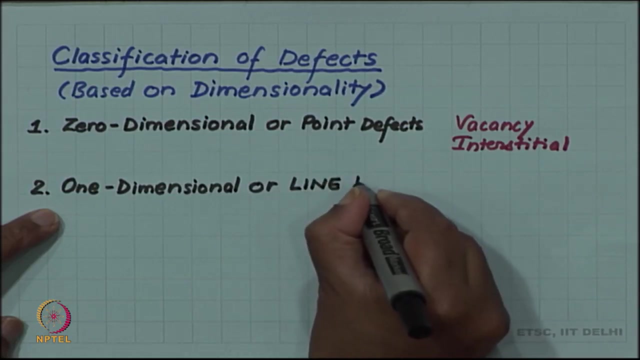 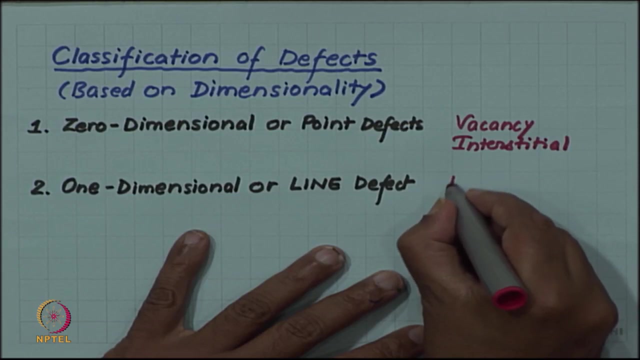 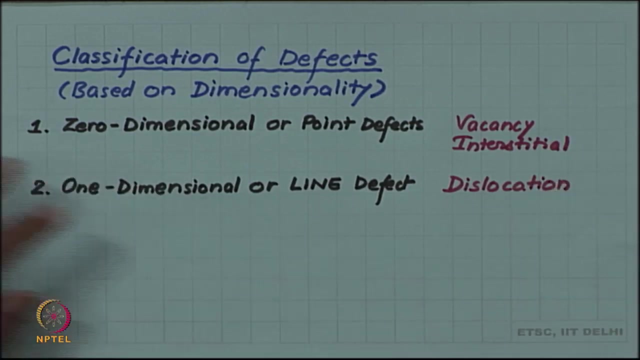 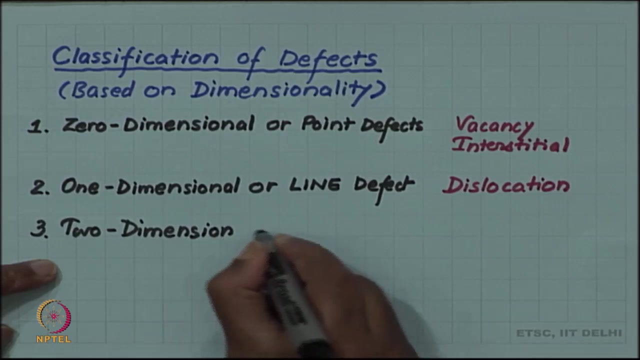 Interstitial, Interstitial, Interstitial, Interstitial defect we can have. we can have one dimensional or line defect and the example will be: dislocation, Dislocation, Dislocation, No, no, no, no. we can have two dimensional. 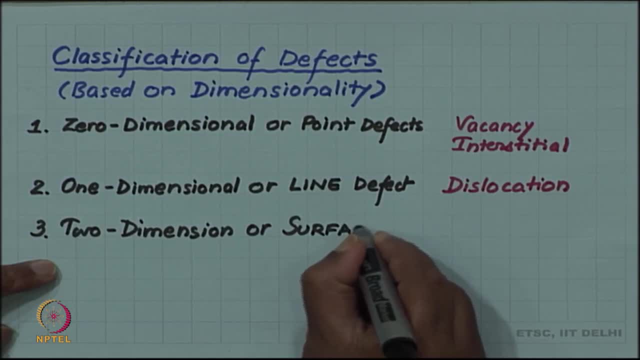 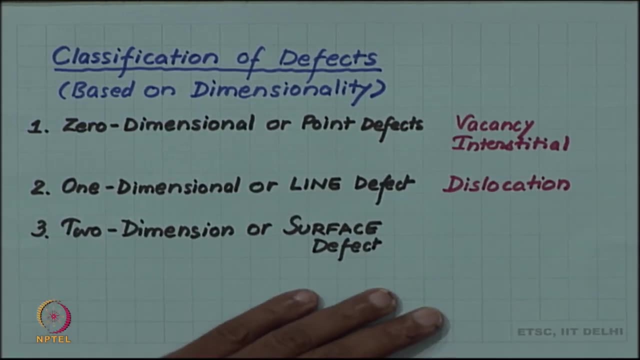 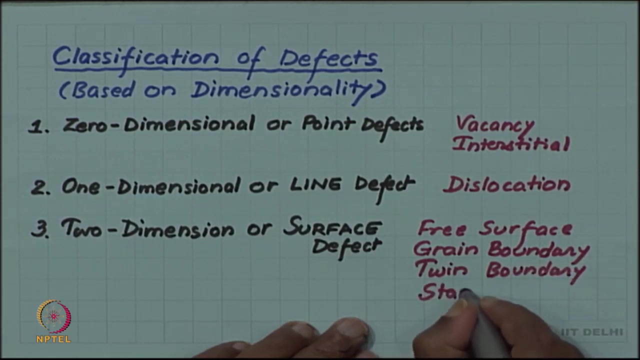 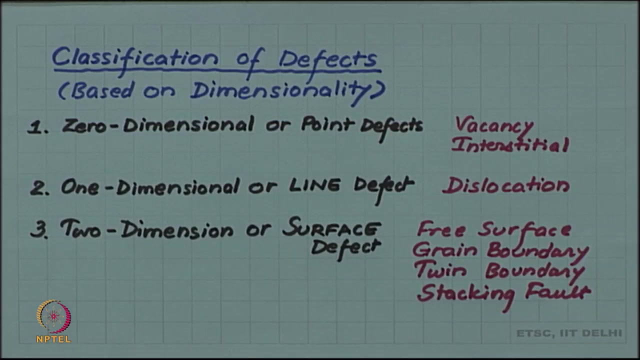 for surface defect, and some examples will be free: surface grain, boundary, boundary, stacking fault. all these are examples of surface defect, So we will look at all these. whatever examples are listed here, we will look at them in detail, one by one. 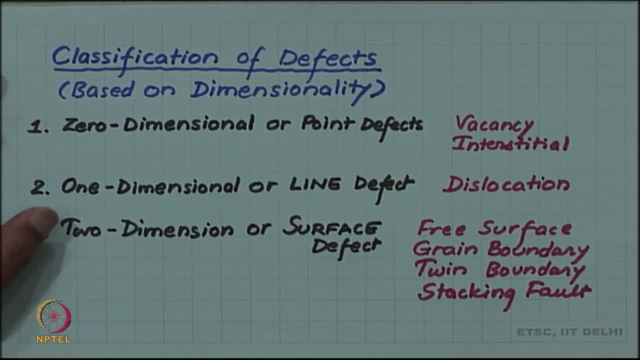 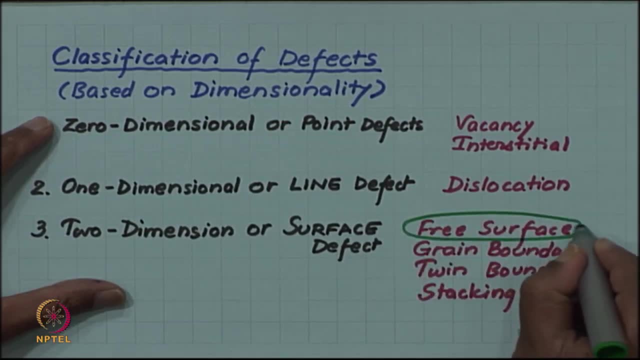 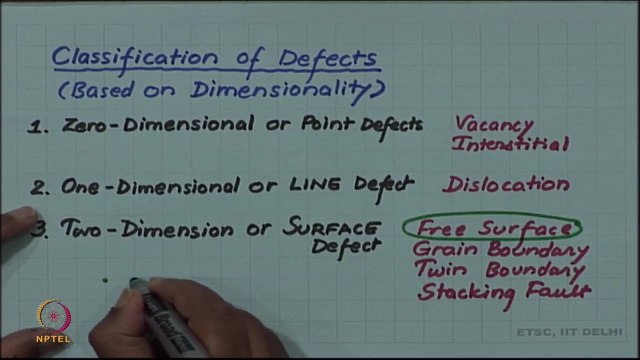 One may think that, why the crystals are not ideal? why do they have defect? First of all, one defect: this free surface will always be present in the crystal, because our crystals are finite and the definition of periodicity requires an infinite crystal, since all lattice. 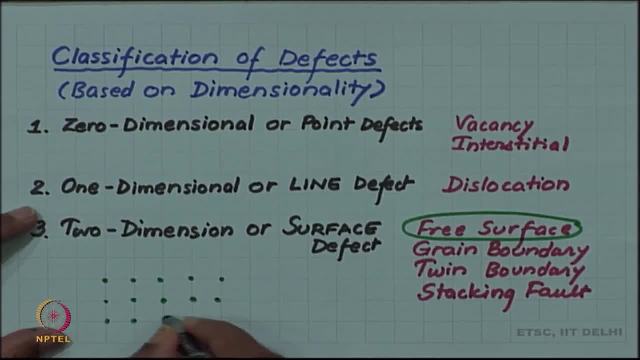 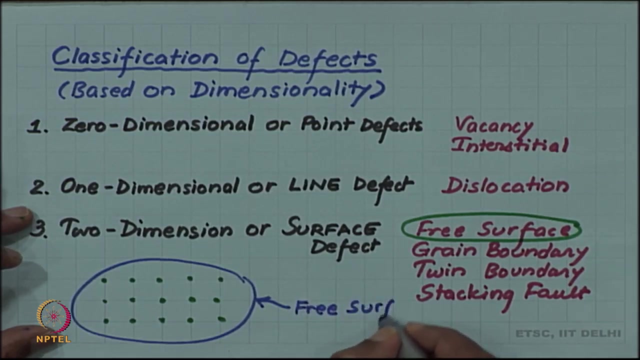 points have to be identical. they cannot be any surface. So the very fact that the crystal is bounded by a surface- because our real crystals will always be a finite crystal- So it will have a boundary line and that boundary or the external surface. that is why we are calling it a defect, because it may appear that, why it should be. 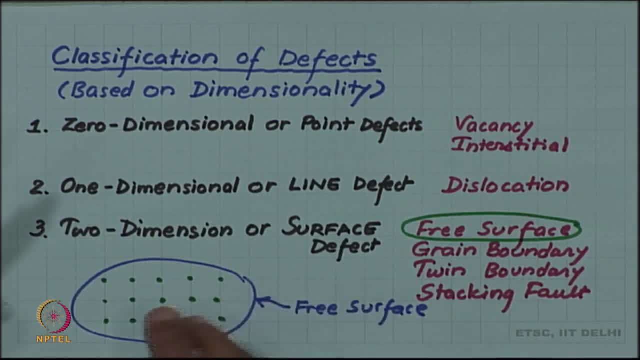 a free surface- a defect, But a free, since by definition of periodicity of ideal crystal the requirement is of an infinite lattice. So only infinite lattice can be an ideal lattice. any boundary will break the periodicity and free surface breaks this periodicity. 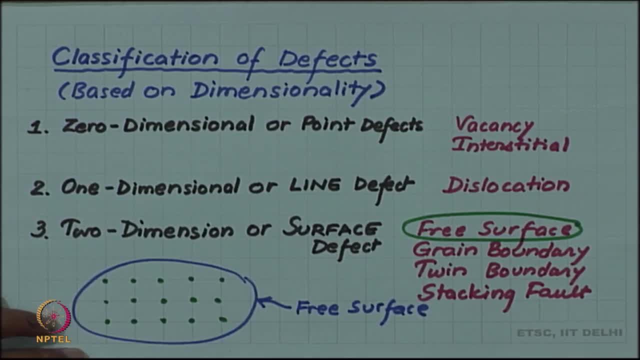 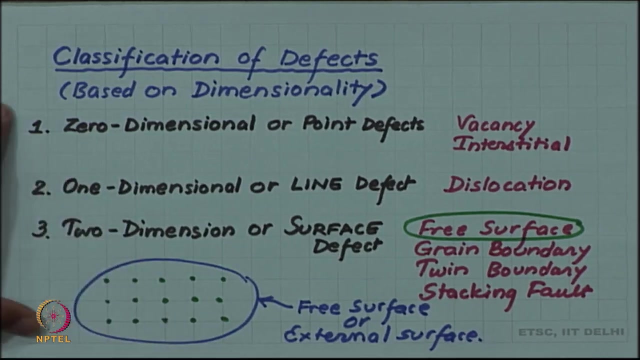 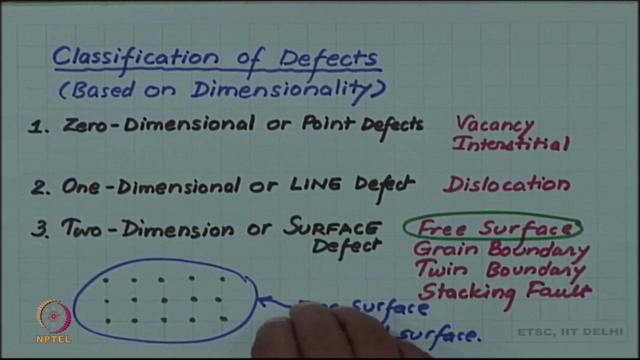 And so the free surface, or sometimes called external surface, will always be present in any crystal, However perfect it is internally. this external surface will always be present in a real crystal. So we will now look at a one by one, these defects as we go along.